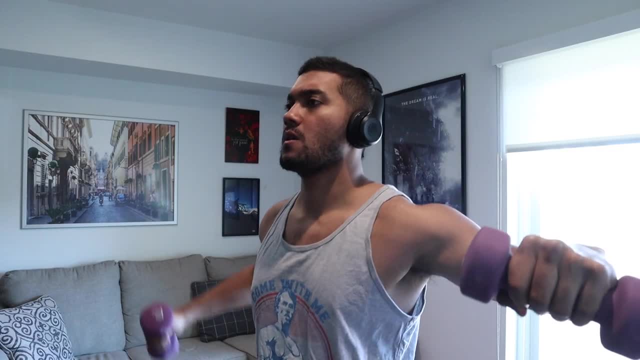 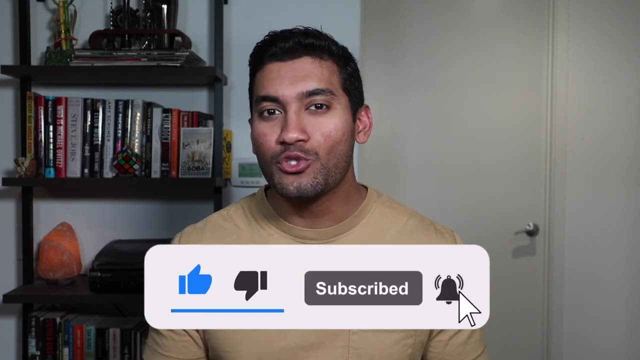 to emails, shopping for groceries or getting enough exercise. It can feel like we're solely striving to work our way through a checklist without assessing whether the stuff that we are doing has any true effect on our goals or long-term plans. This is where personal development expert Brian Tracy comes in. 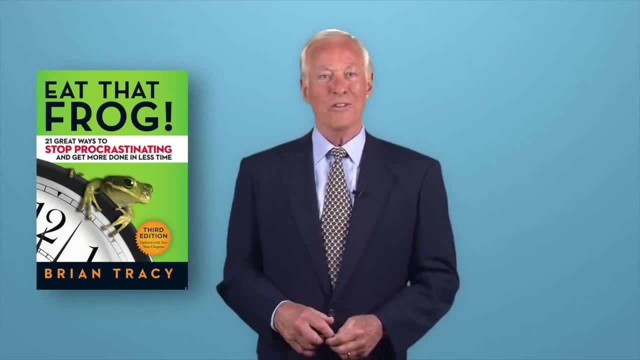 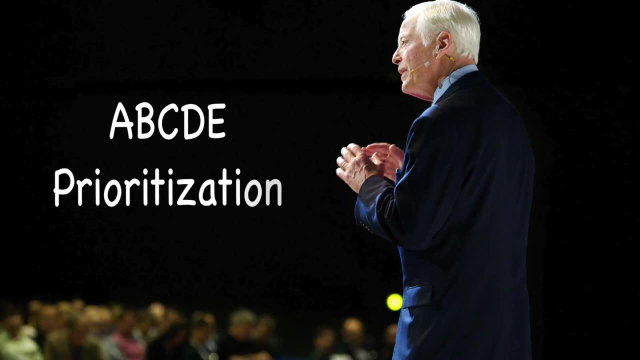 Tracy is best known for his book Eat That Frog, a technique to stop procrastinating and get things done. But where I believe he stands out is his practical approach to prioritization, called the ABCDE method. It works like this: Grab yourself a piece of paper and list out. 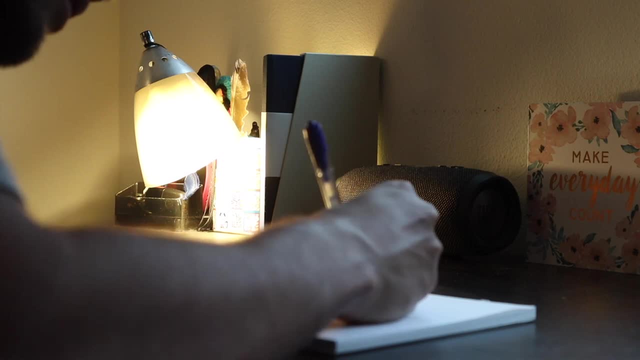 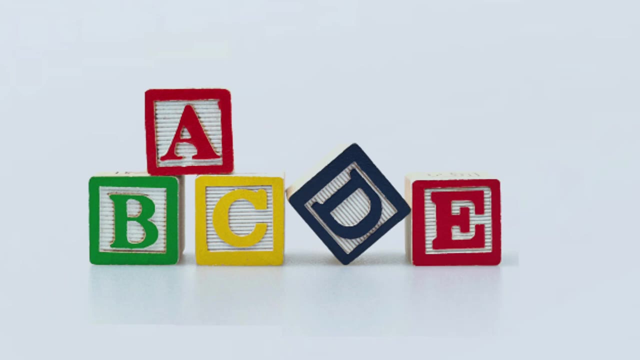 all the tasks that you need to complete. Once that's done, you'll need to go back to your worksheet to begin assigning the letters A, B, C, D and E to your tasks, depending on their level of importance and priority. A includes items that are the most important. These bring you closer to your goals and you 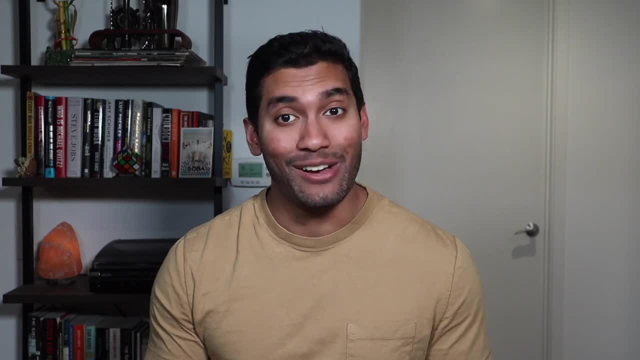 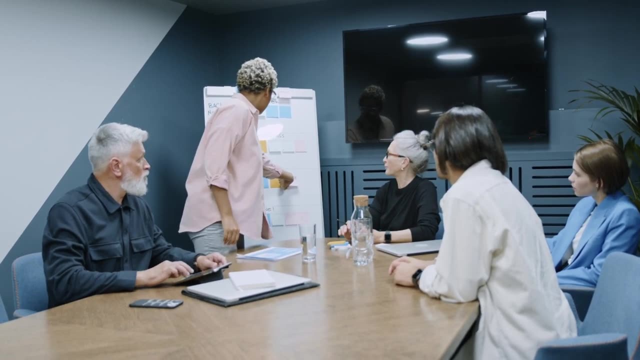 cannot avoid them. There also tends to be a potentially grand downside should you not complete them. This could be work that might affect a client or that your boss is asking for and you want to try to limit this to about 3 items. List them as A1,, A2, and A3 in order. 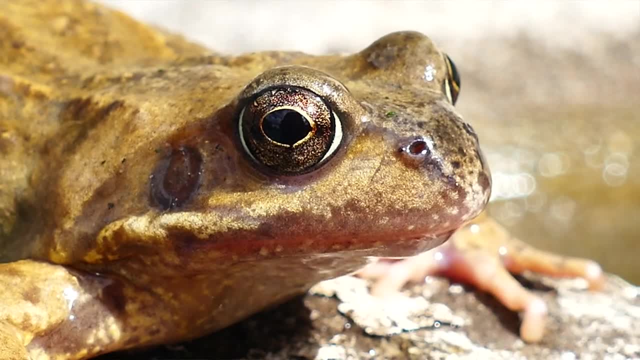 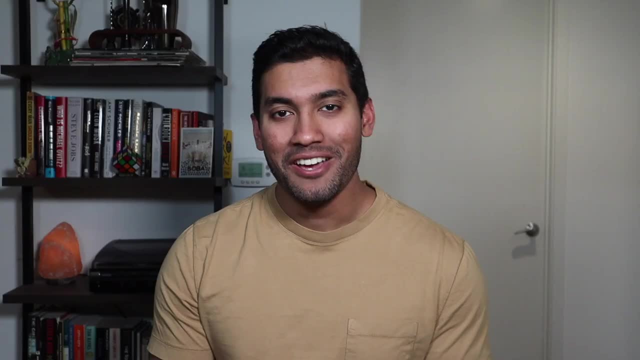 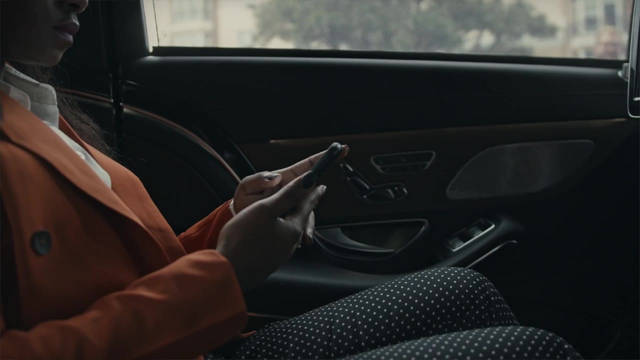 of priority B includes items that you should do but have relatively minor consequences. The rule that you should follow is that you never do a B task before all the A tasks have been completed. Generally, this tends to be items like returning phone calls or replying to emails. 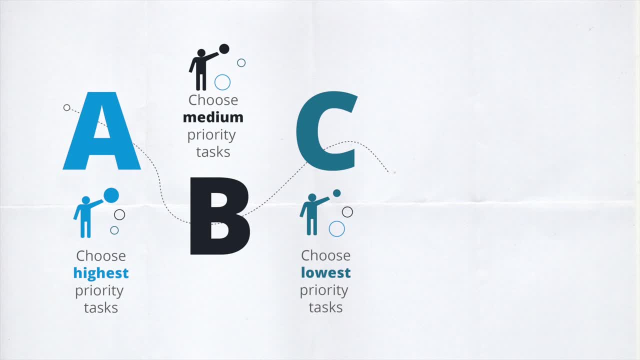 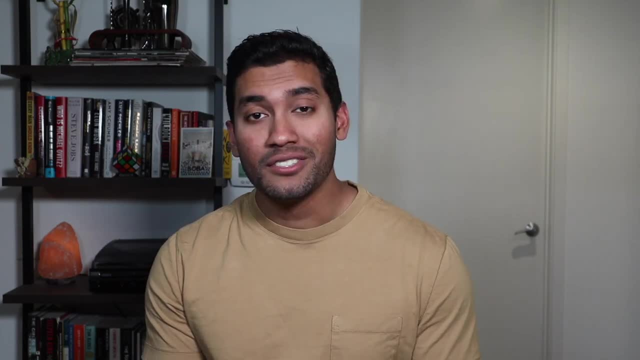 C tasks are those that you'd probably want to get done and do not have any consequences. You don't want to leave these out, but they're generally not related to your work or your goals, So this could be things like running errands or grabbing lunch with a friend. 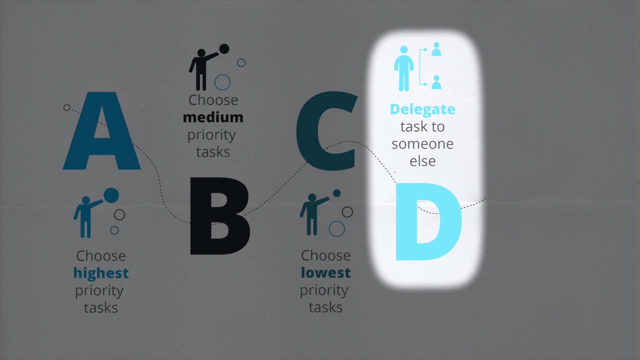 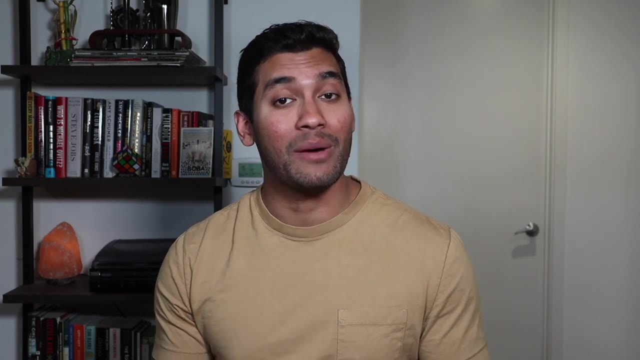 Next are D tasks. So this is the category where you're hoping to delegate to someone else in order for you to focus on more important items in your A category. A good way to think about this is figuring out whether someone else could handle it with a quick explanation. 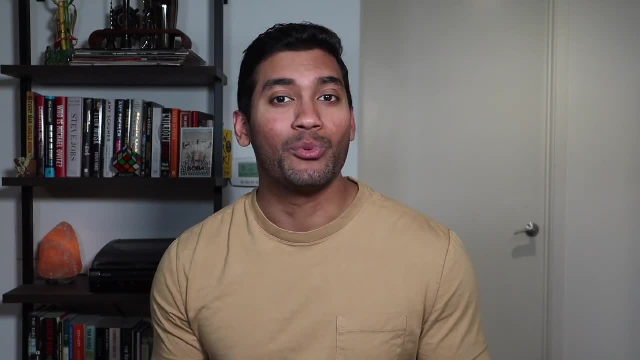 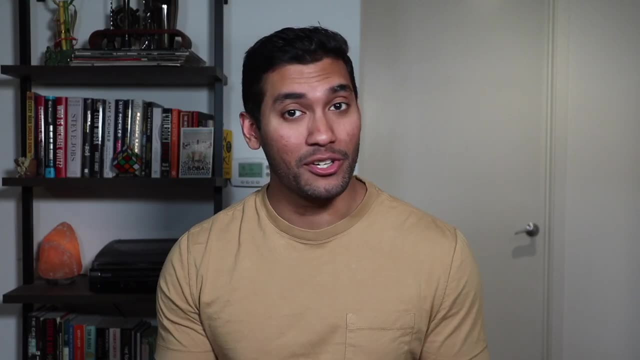 or whether it's technically someone else's job. This is simply about resource allocation to help you focus better. Finally, there are E tasks. An E activity should ideally be eliminated. It's a good opportunity for you to audit your tasks and identify whether you really need to do everything on your